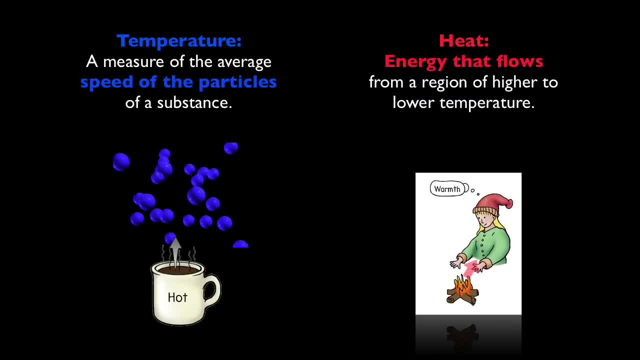 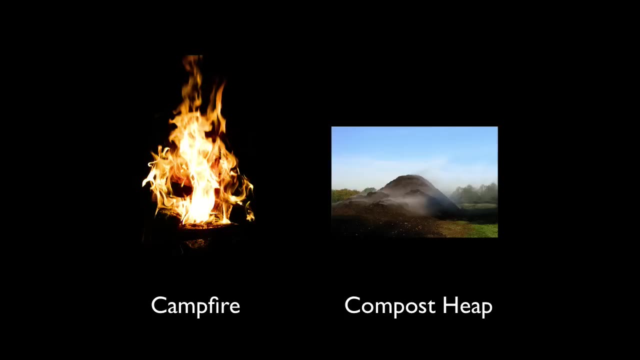 concepts you should hopefully recall from your study of physics. Well, now's the time where you're going to see some amazing application of these very concepts. Let's take this step-by-step, starting with an analogy. Which has a higher temperature? a campfire or a warm compost heap? 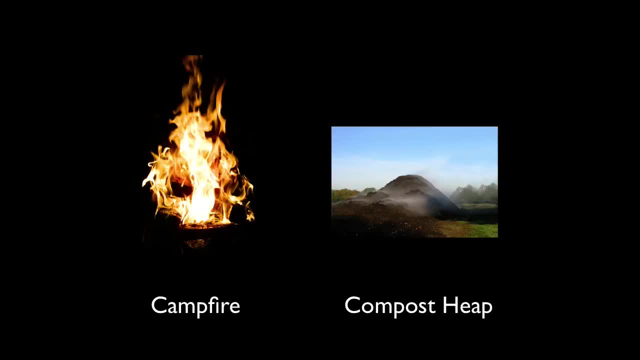 Indeed, the campfire, which is to say the average speed of the atoms in the campfire, is much faster. That's why you wouldn't want to put your finger in the campfire. But the campfire and the compost heap are both releasing energy to the environment, right? The campfire releases it real quickly. 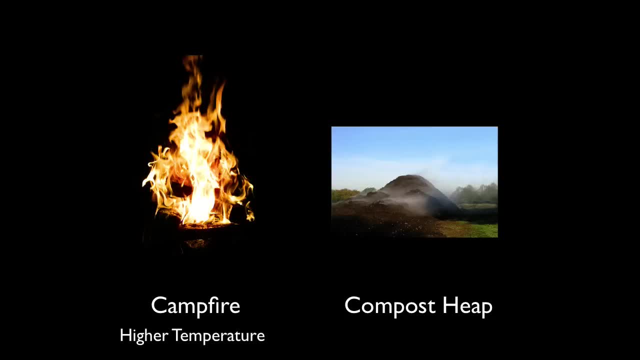 because of its higher temperature, And the compost heap releases energy much more slowly because of its lower temperature. Got that. Now what if the compost heap were much bigger? Say, it has the very same temperature, but it's much, much bigger, like the size of many city. 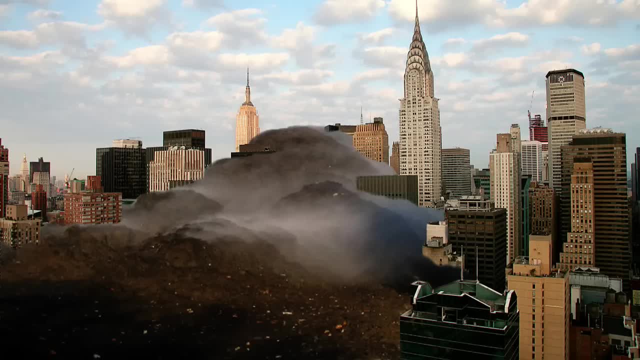 blocks Because of the temperature. it's much, much bigger And the compost heap releases energy because it's bigger. Do you see that the total amount of energy it releases each second is also much bigger? Any bit of the compost heap might not be that much, but add it all together and wow. 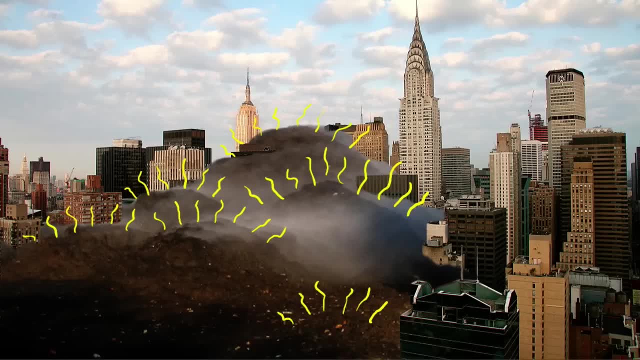 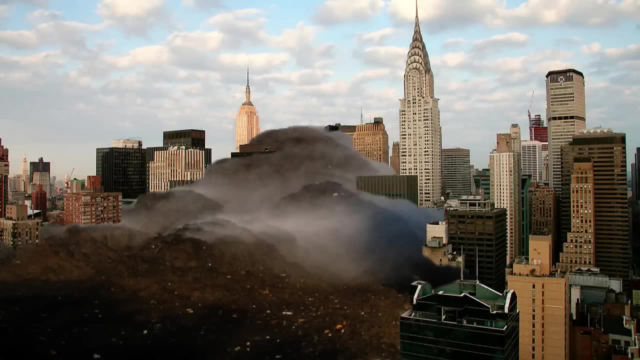 that's a lot of energy. So let me ask you which releases more energy: the small campfire or this humongous compost heap? Sure, the campfire has a higher temperature, but it's quite small by comparison. So you see, this lower temperature compost heap puts out much more total energy than the higher. 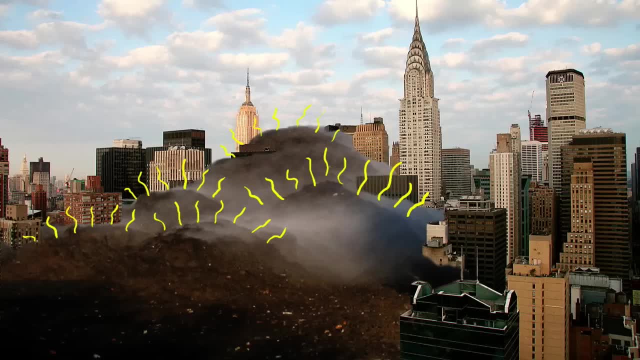 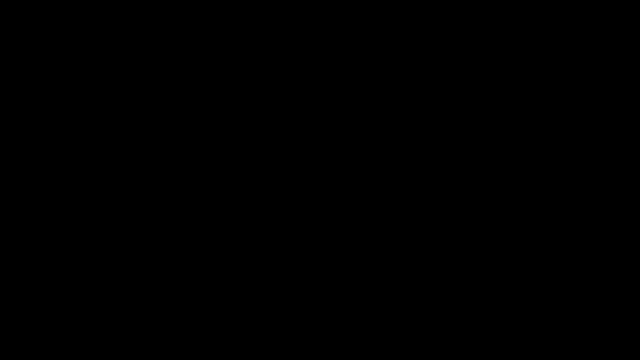 temperature. campfire Temperature and heat are not the same thing. If you understand this, you'll understand the same thing happening with stars. The star Procyon has a toasty surface temperature of about 6,500 Kelvin. Remember, we get the surface temperature from the star's color. 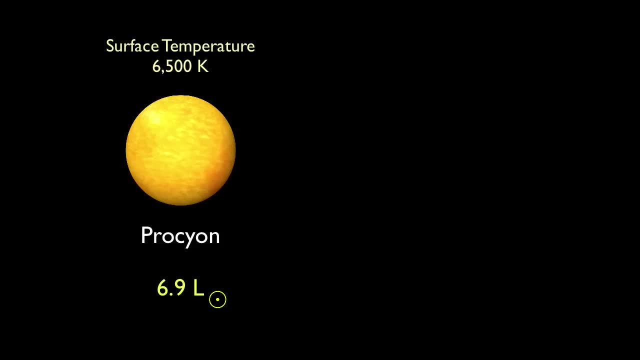 Its luminosity is a mere 6.9.. Oh, and remember from the last lesson that luminosity is a measure of a star's energy output relative to our own sun. So Procyon is 6.9 times more luminous than our sun. 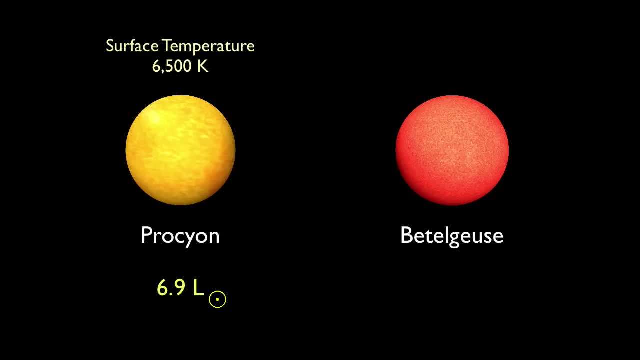 Okay, The star Betelgeuse has a surface temperature of about 3,000 Kelvin, So because it's cooler, you might expect its luminosity to be less than 6.9, huh, Well, that might be true if they were the same size as shown here, But that cool-to-the-touch Betelgeuse 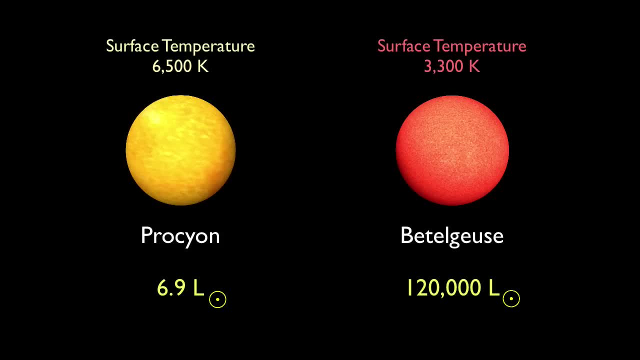 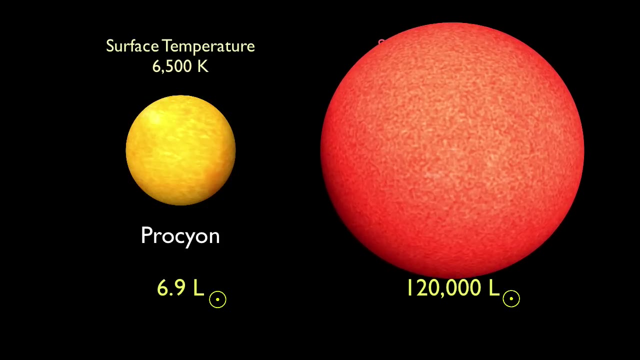 has a luminosity of about 120,000.. Huh, How can something this cool put out so much energy? Think of the compost heap. Your conclusion: Yeah, They obviously cannot be the same size. That Betelgeuse puts out so much energy and is yet cooler. 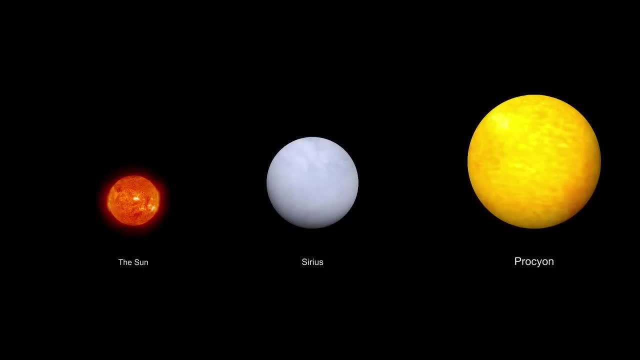 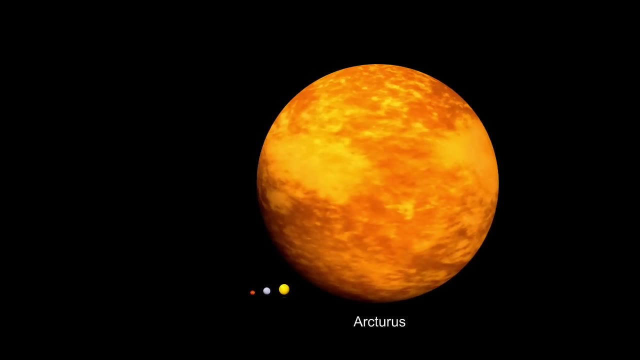 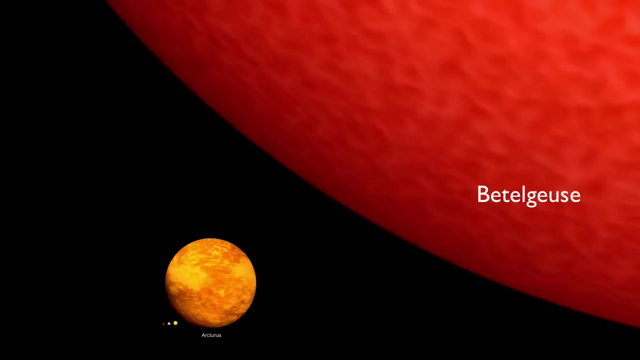 It tells us that Betelgeuse must be much larger, A luminosity of 120,000?. Betelgeuse must be extremely large. Indeed, the calculations made by astronomers show Betelgeuse to be astoundingly large. The point here is that by comparing the luminosity of a star to its surface temperature, we gain. 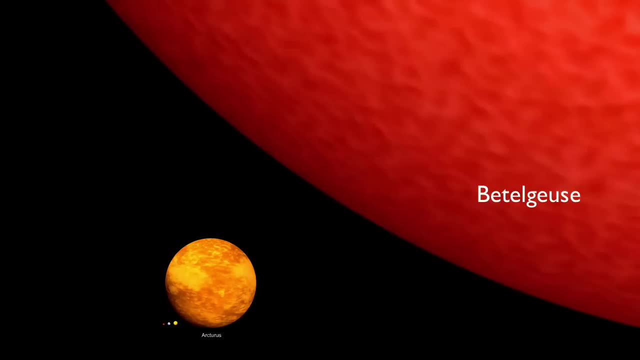 a measure of that star's size. Now, that's crafty, Because it means we don't have to actually travel to a star in order to measure how big it is. It also allows us to study and compare stars to each other. In doing this, we can get a sense of all the different. 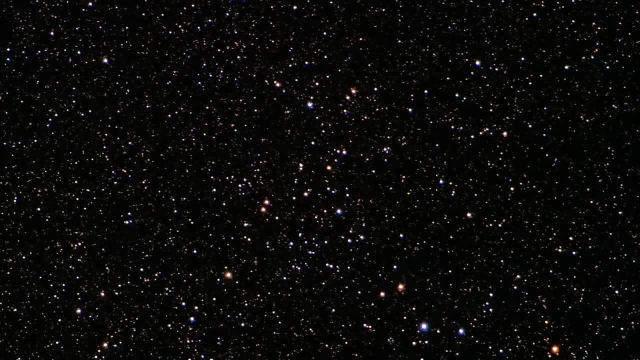 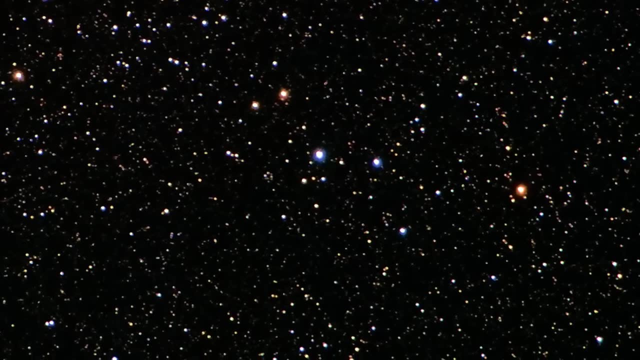 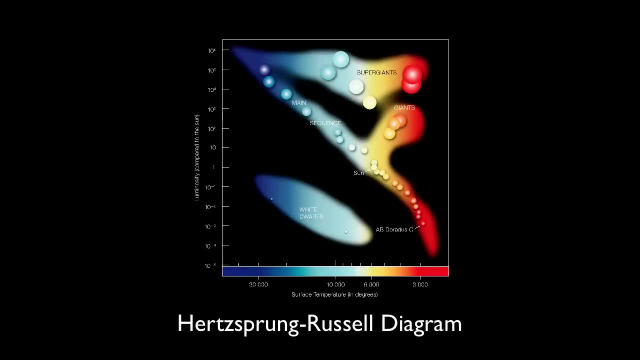 kinds of stars there are. This in turn allows us to reveal the potential histories and life cycles of stars. The graph that correlates stellar luminosity to temperature is called the Hertzsprung Russell diagram, or the HR diagram for short. It's a rather important diagram In many ways. 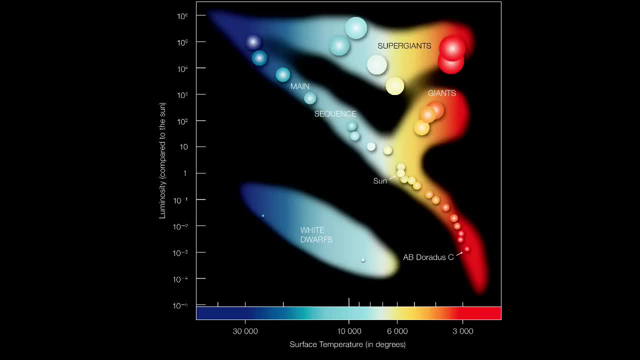 what the periodic table is to chemistry, the HR diagram is to astronomy. As a chemist myself, I like to call it the periodic table of astronomy. Of course, don't memorize this thing. Rather, let's learn how to read it. Luminous stars are at the top and dim stars toward. 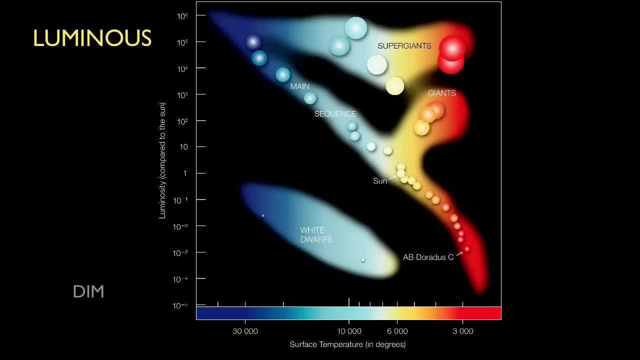 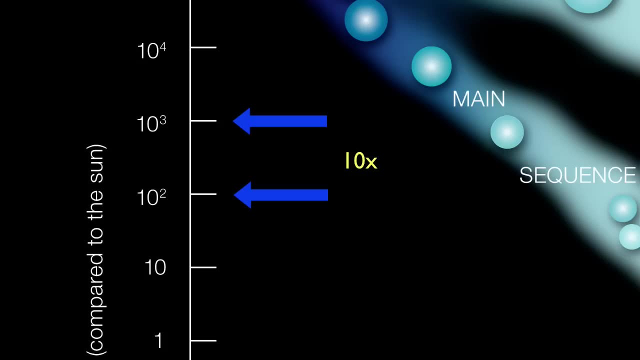 the bottom. Note that luminosity is given in exponents. For example, when you go from here to here, the luminosity is 10 times as great From here to here. you're talking about a hundredfold increase in luminosity On the horizontal axis- the higher surface temperatures. 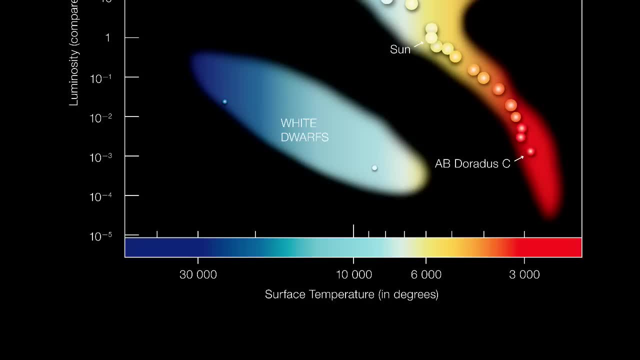 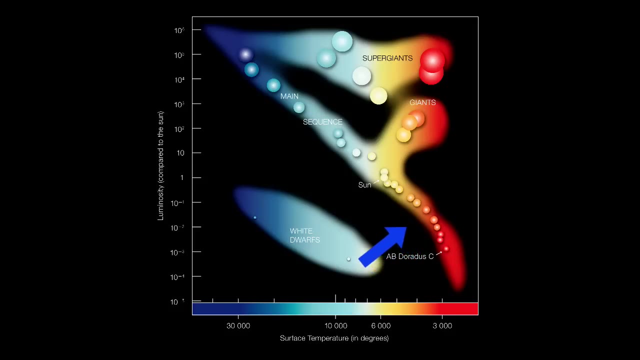 are shown to the left. Anything about 10,000 Kelvin or greater is indicated as a bluish star. Anything cooler than 4,000 Kelvin is shown as a reddish star. Most stars fall within a diagonal line, which we call the main sequence. Our sun is an example of a main sequence star. 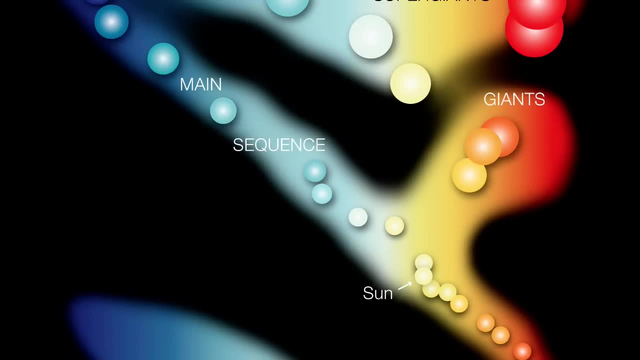 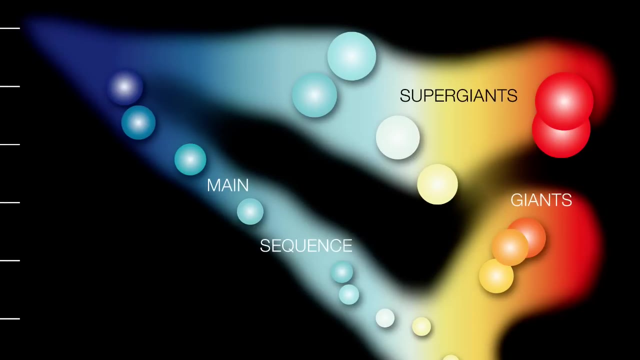 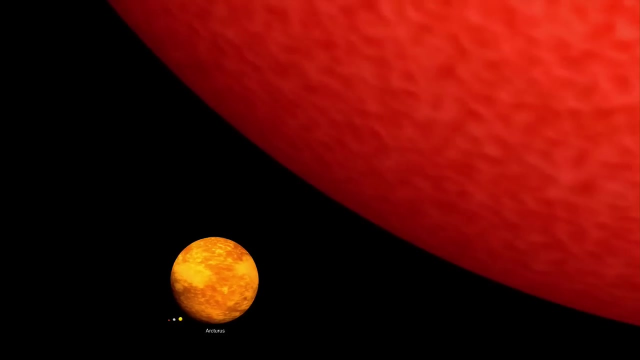 All these stars are burning primarily hydrogen as their nuclear fuel. Above the main sequence are the giants, supergiants and even the hypergiants. Here, Arcturus is an example of a giant, Betelgeuse is a supergiant. Well, maybe a hypergiant. It's subjective, But VY. 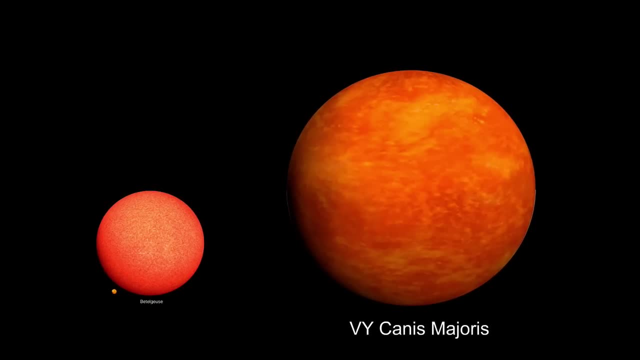 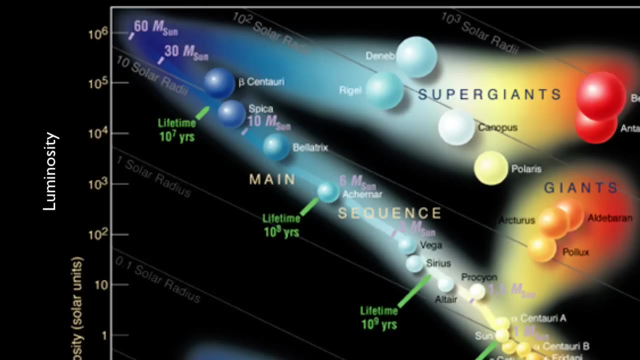 Kenes Majoris. now that would definitely be a hypergiant. The HR diagram plots luminosity using exponents. It has to, Otherwise the range of luminosities wouldn't fit on a regular-sized piece of paper. Likewise, it's not very practical depicting the relative sizes of stars on a 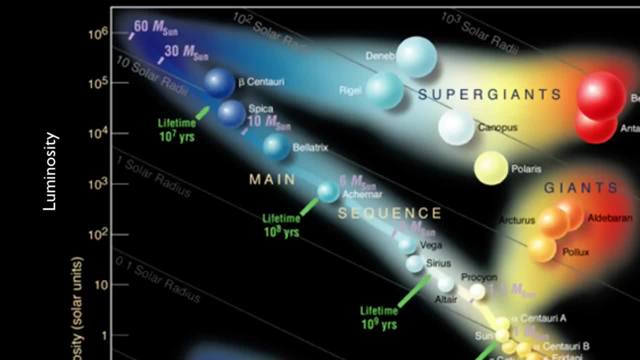 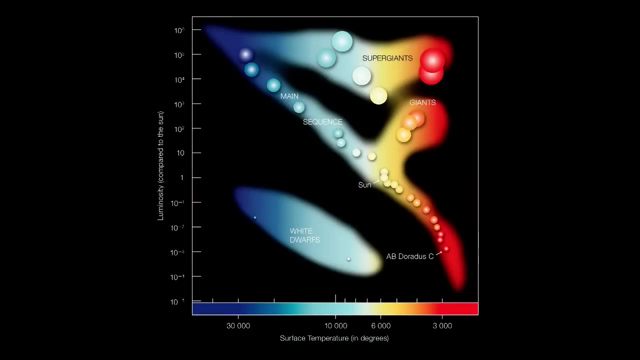 regular piece of paper. Even our diagrams, when printed on regular paper, are limited in their ability to give us the sense of star sizes, But here in video, we don't have that limitation. Nice, eh, Oh, we should talk about densities. Get this As large as Betelgeuse is. it's only about. 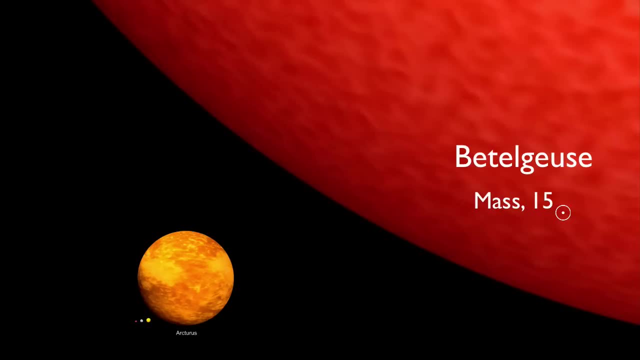 15 times more massive than our sun. So while it's huge, it's only huge at the expense of not being very dense. Its outer photosphere, for example, is less dense than the air you're breathing right now. That's billions of times less dense than our much smaller but much more compact sun. 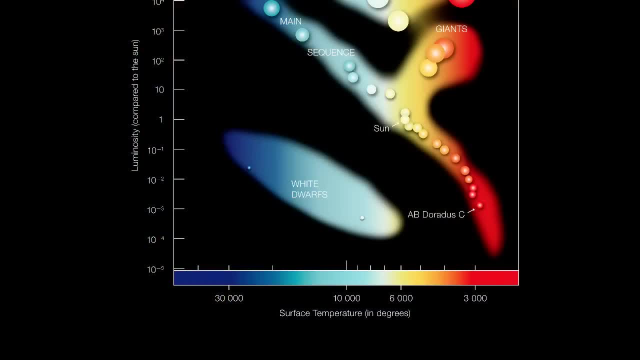 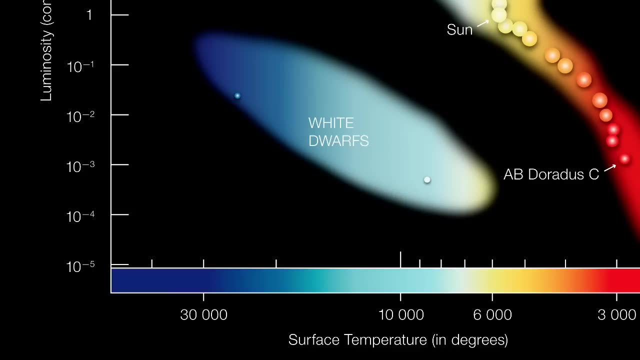 Speaking of compact, below the main sequence, we have stars that are necessarily tiny. This includes the white dwarfs. We'll be talking about white dwarfs in more detail in a bit. Briefly, our sun is destined to become a white dwarf. 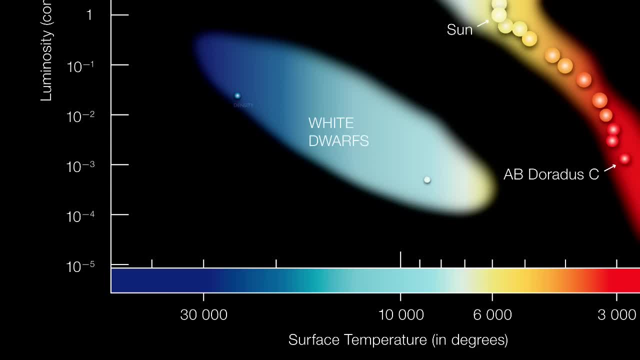 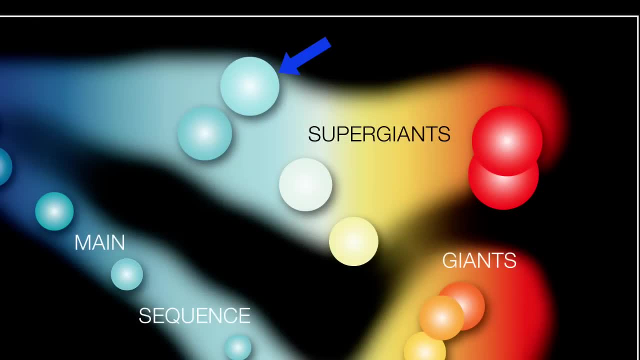 When that happens, it'll have a density that's out the roof, like a million times that of gold. Oh, what's the difference between a blue supergiant and a red supergiant? Well, one has a higher temperature, right. 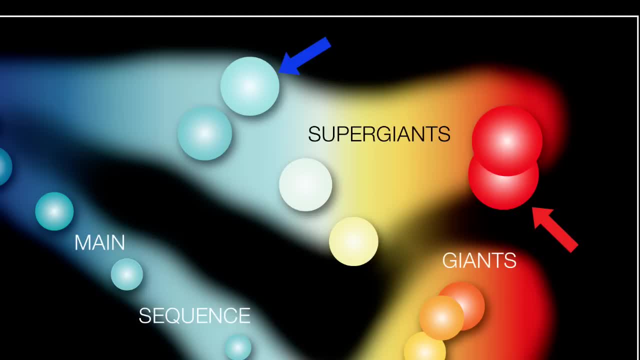 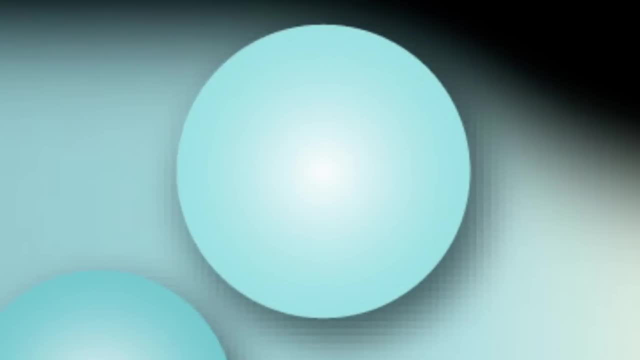 Which Good. But why might the blue supergiant have a higher temperature? Oh, it must be cranking out more thermonuclear fusion. So which do you suppose would be more dense, a blue supergiant or a red supergiant? 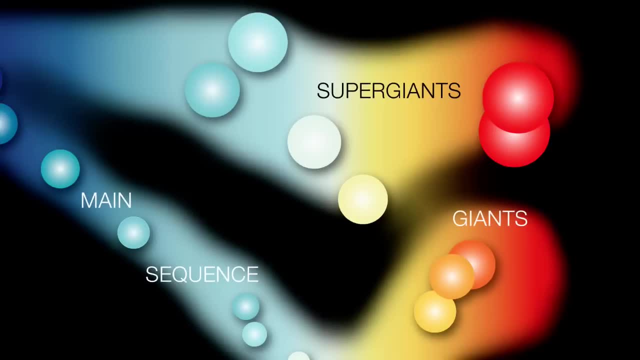 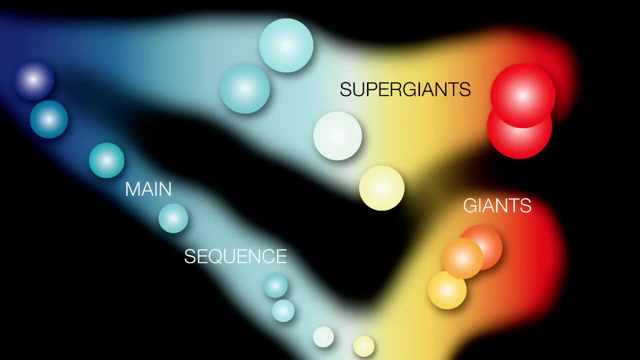 If you're going to have more thermonuclear fusion, you're going to need a good concentration of fuel, right? So the blue one, Hey, excellent. Hmm, You might even be in a position now to answer why it is that the 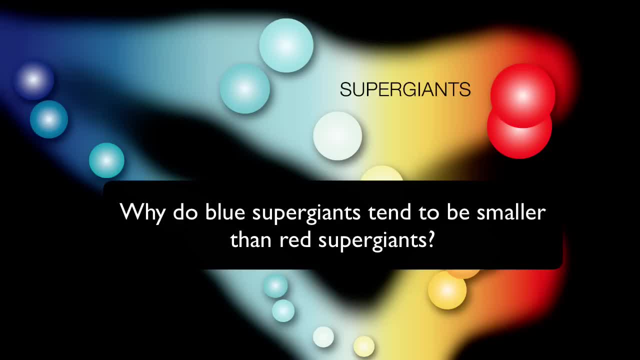 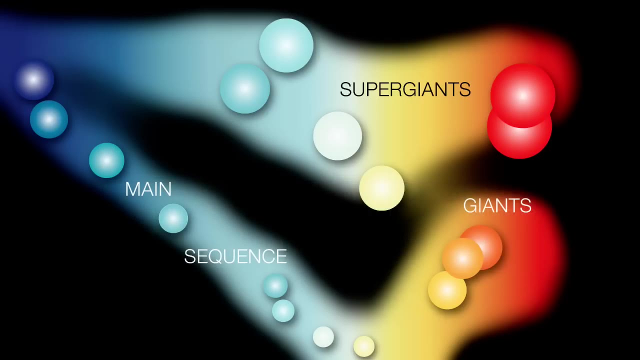 average blue supergiant is smaller than the average red supergiant. How nice if you could talk about these and other questions with classmates or, better yet, with classmates and your course instructor all together in the classroom. Don't think that you're going to have command over these concepts just by watching these. 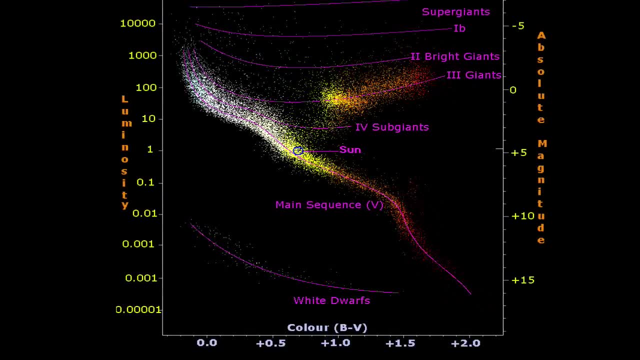 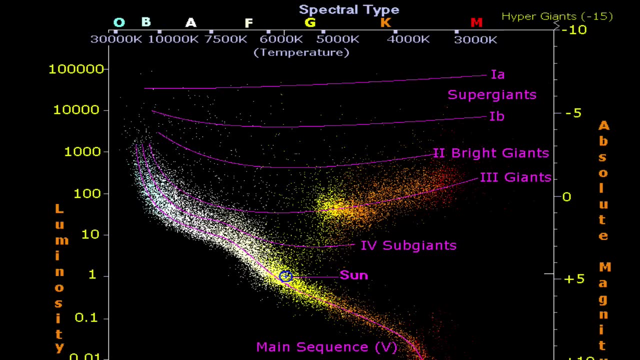 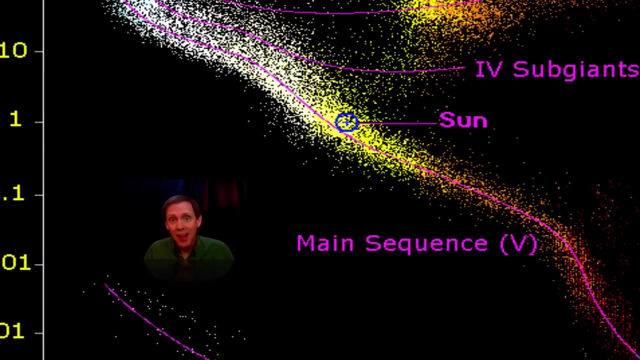 videos over and over again. No, you need to try articulating these concepts yourself. If you want entertainment, just sit back, relax and watch, like you might do at some sporting event, Subtitles by the Amaraorg community. That's not bad. We all appreciate good entertainment. All I'm saying is, if you want to be a player, 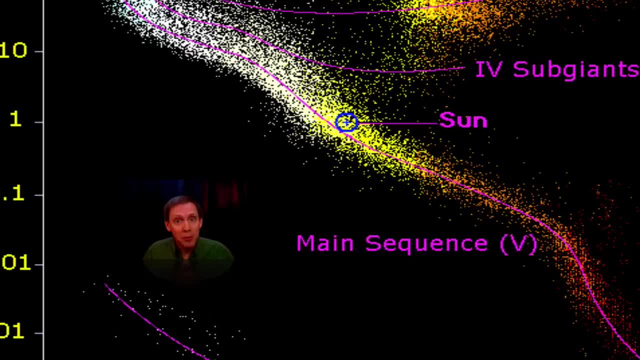 you got to play. If you want to do well on your exams, you got to do more than just watch. You got to interact. You got to get your mouth moving. Are we interacting? No, I'm just lecturing to you and you're listening. That's not good enough.